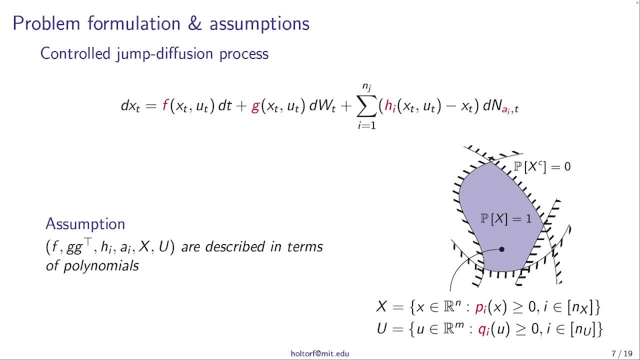 some integer lattice or something of that sort, and I will critically assume that everything about the process is described in one way or another in terms of polynomials. So, in particular, for all the functions that characterize the dynamics of the process will be assumed to be a polynomial. 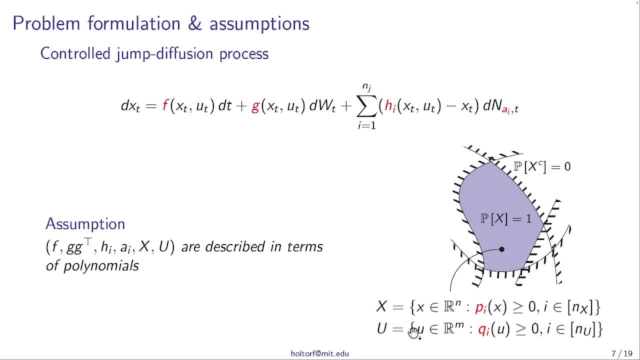 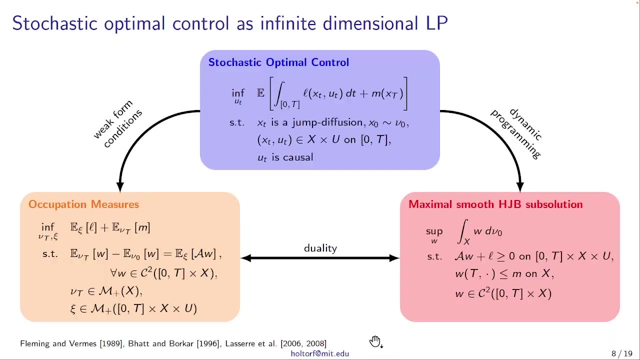 both jointly in the state and the control action, and also the state space and the set of admissible control actions are both assumed to be basic closed semi-algebraic sets. So sadly I don't have time to go into the theoretical details of all this, but what I believe is worth mentioning is that these 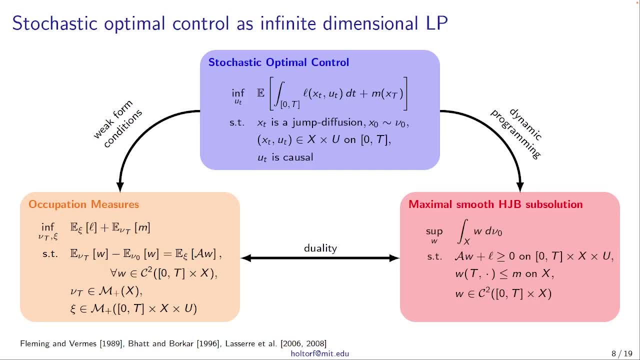 types of stochastic optimal control problems are under technical assumptions equivalent and in practice, anecdotally speaking, often very well approximated by a primal dual pair of linear and or infinite dimensional linear programs. And today I want to really focus on this sort of dynamic programming route here on the on the right, So don't worry too much about the notational. 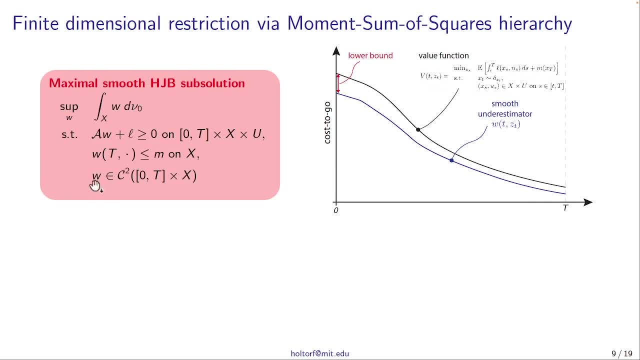 details here. all that the problem on the left is saying is that we are looking for a smooth function w which underestimates the value function of the cost to go associated with the original optimal control problem and, in particular, we are looking for that smooth function which under-approximates. 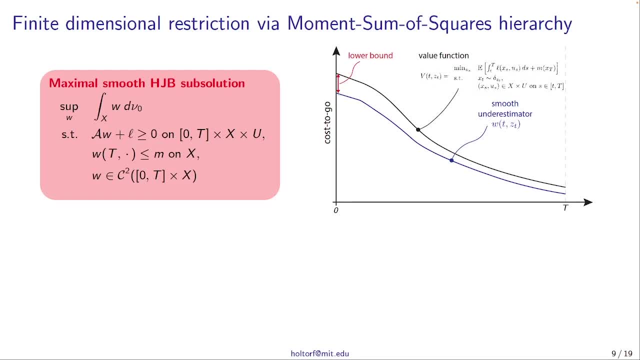 this value function as best as possible at the initial time, and from there it will be easy to convince yourselves that we are in fact controlling the state space of the process. So let's look at how to construct a hard-limit bound on the optimal value of the stochastic optimal control problem. 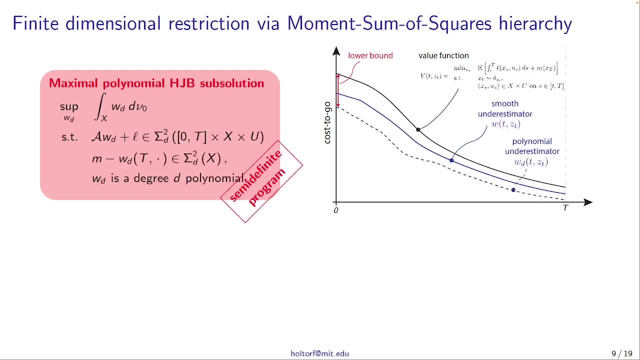 But of course this is still a super hard problem to solve. so we can utilize sort of the magic of the moment sum of squares hierarchy to construct tractable restrictions, usually in the form of semi-definite programs, simply by optimizing over some fixed degree polynomial as opposed to. 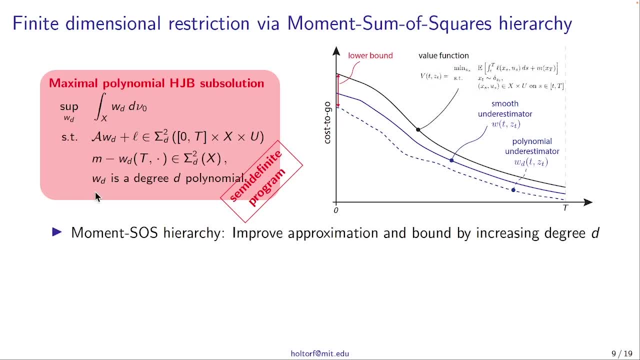 any smooth function, And then we can trade off more computation for better bounds and better approximation, simply by increasing the degree of that polynomial. A nice thing about this approach is that it provides us with an approximate value function that then down the line can inform controller design. But- and I think anyone who's ever used these kinds of things in 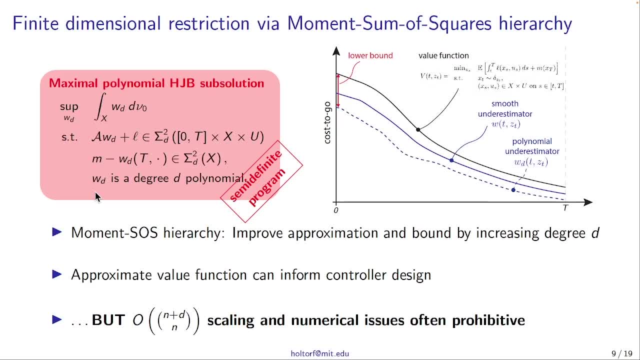 practice will agree with me. it's actually quite limited. In particular, the scaling isn't great and, more importantly, numerical issues are often prohibitive. So in practice, we can often only do this for moderate degree polynomials, which may not be good enough to give us informative 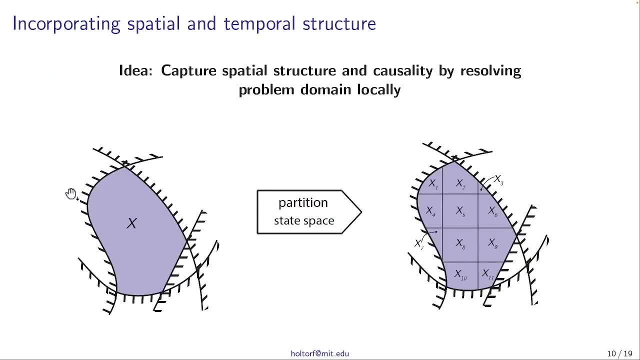 bounds. So one way to kind of sidestep that issue, which in my opinion is criminally neglected in the literature, is to use a single-digit number function to calculate the number of arguments. So in the least we can use a single-digit number function to calculate the number of arguments. So in the 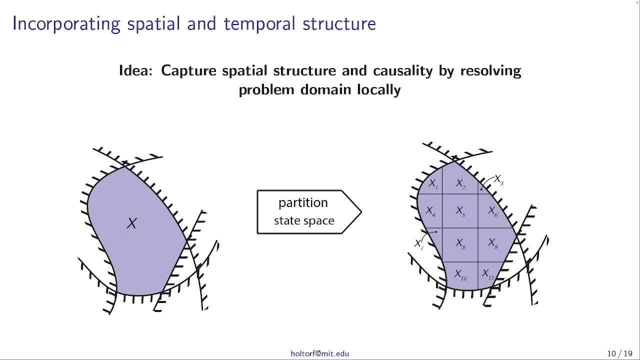 that we can actually weaken our restrictions, not only by increasing the degree of the polynomials that we optimize over, but instead look for a piecewise polynomial underestimator. So, in particular, we can partition the state space as shown with these tiles here: 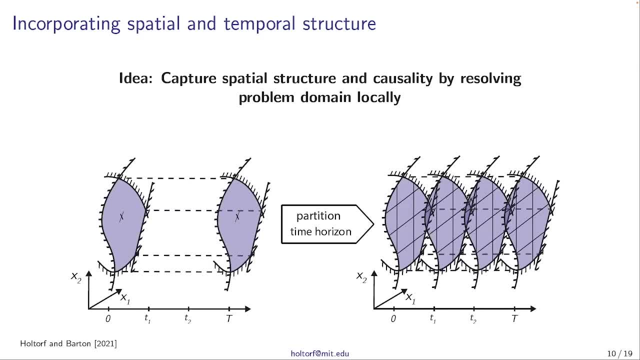 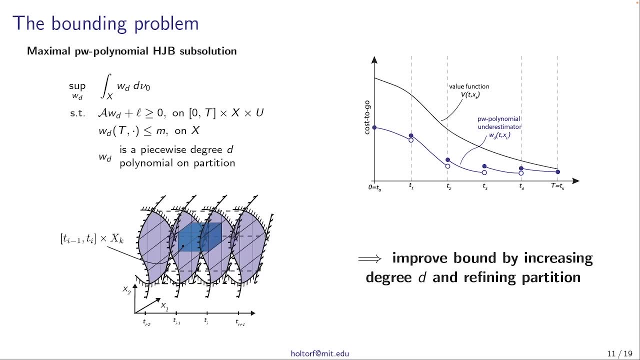 as well as the control horizon of the problem, to then get a partition of the whole problem domain, which is the product of the control horizon and the state space, and then write out a problem which looks very similar, but instead of looking for a polynomial. 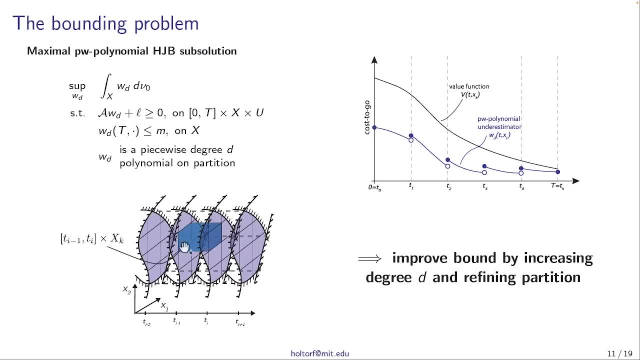 we are now looking for a piecewise polynomial, where each piece is defined on such a subdomain of this partition And then the output is of course some piecewise polynomial underestimator of the value function. So then we can improve the approximation quality. 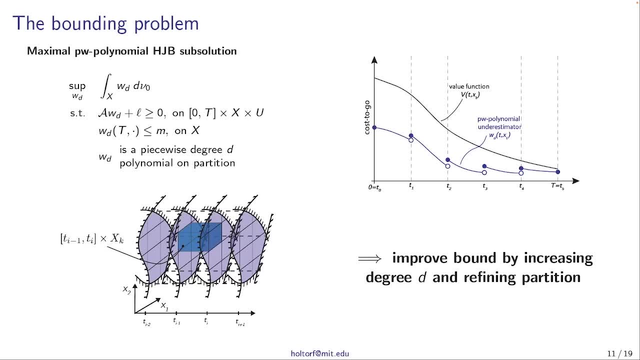 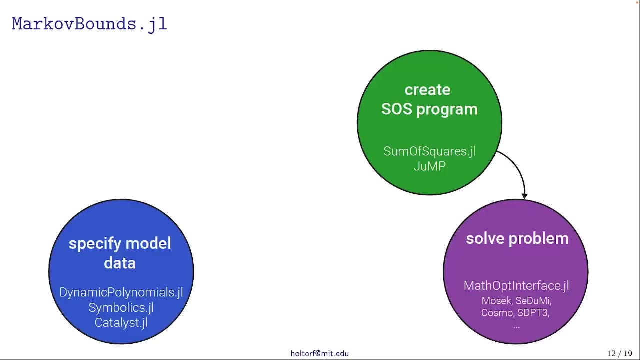 of this problem here, not only by increasing the degree of the polynomial pieces, but also by simply refining the partition. And while this does not offer any inherently better scaling in principle, it turns out to be quite advantageous in practice in many cases. So where does MarkovBoundsjl now fit into all of this? 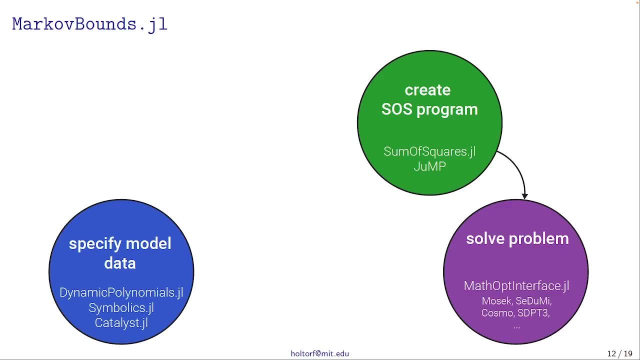 So the nice thing is that the Julia ecosystem in principle already supports everything that you need in order to set up and solve these types of problems. On the one hand side, we have very powerful symbolic modeling tools that allow us to specify our model data quite conveniently. 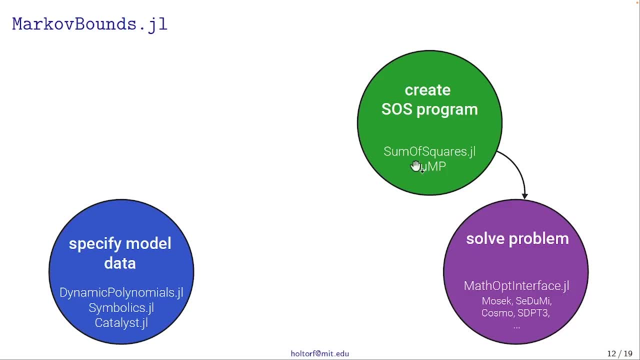 And, on the other hand, we have sumofsquaresjl, which allows us to very easily set up sum of squares programs and then push it through the MathOpt interface to our favorite optimizers. However, if you are a practitioner or someone not familiar, 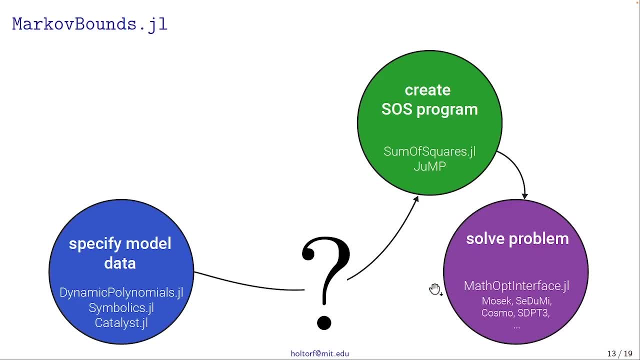 with sum of squares programming. it may not be obvious how to translate this high level problem data to the correct sum of squares programs to be solved And, in fact, even if you are very familiar with these things, it may actually involve a very large amount of bookkeeping. 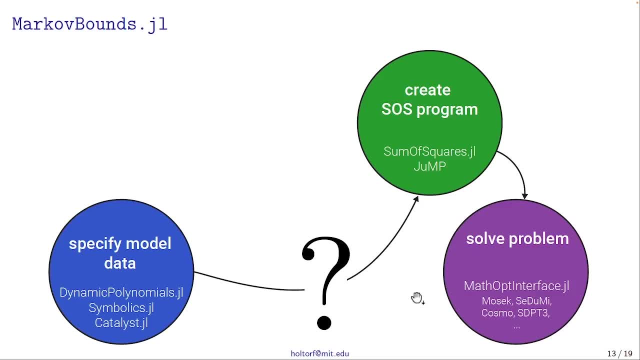 which is error prone, in particular if you go down the route of optimizing over piecewise polynomials. So, and that is a gap that MarkovBoundsjl attempts to fill- The idea is to only take in high level input data and then automate the process. 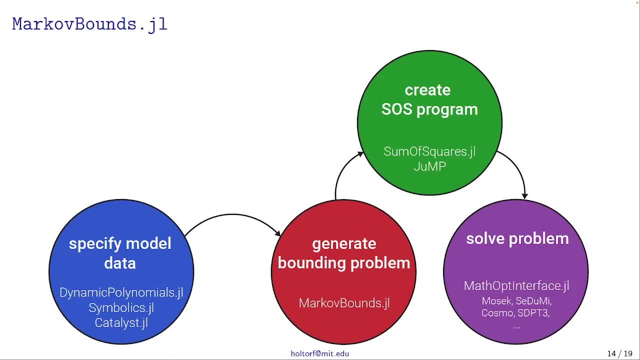 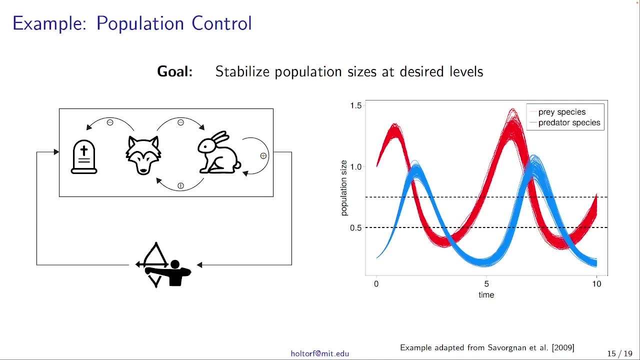 of setting up the correct sum of squares programs and push it through the existing pipeline. So to show you how that may look like, I brought a small example from population control, where we are looking at a noisy environment in which a predator and a prey species 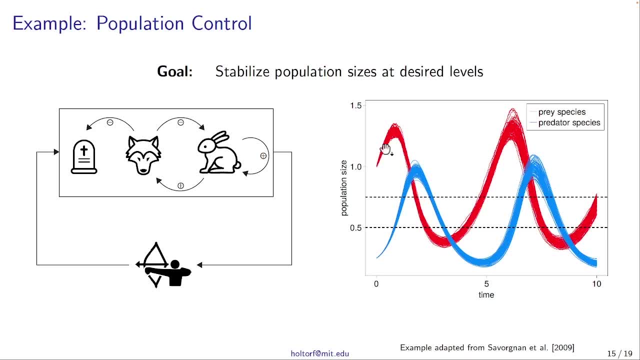 interact with each other And, as long as left uncontrolled, their population sizes would show this oscillatory behavior. here And now, our goal is to regulate the effort of hunting the predator species in a way to drive the population sizes to some stable desired reference value. 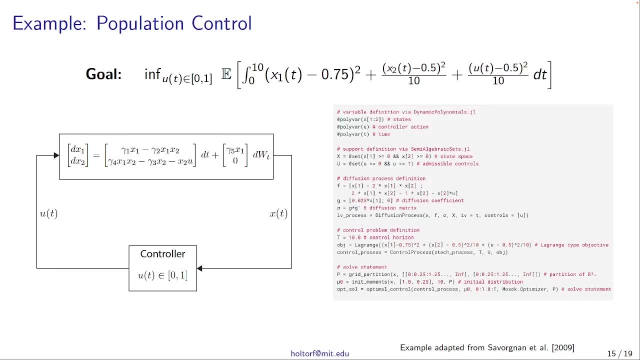 So this whole problem can be modeled as a diffusion problem, a non-linear diffusion process to be controlled, And on the right you see that using MarkovBoundsjl it only takes a few lines of what I would call pretty intuitive syntax. 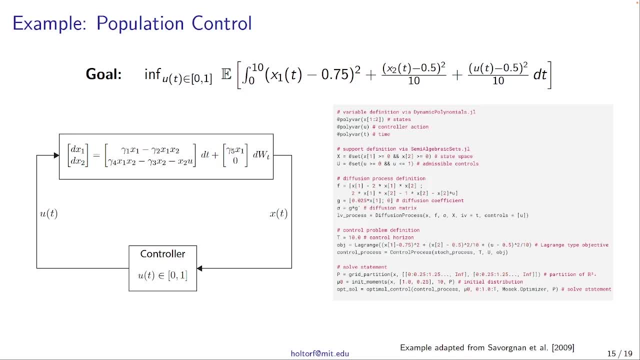 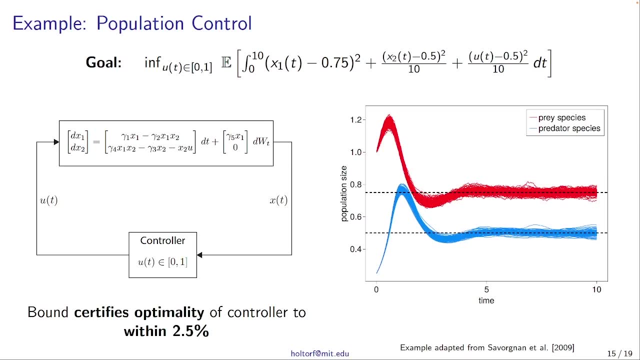 to set up and solve the associated lower bounding problems. So, and to show you that this actually works, what I did is I ran this code and then I constructed a heuristic controller that effectively descends greedily on the approximate value functions that these bounding problems furnish. 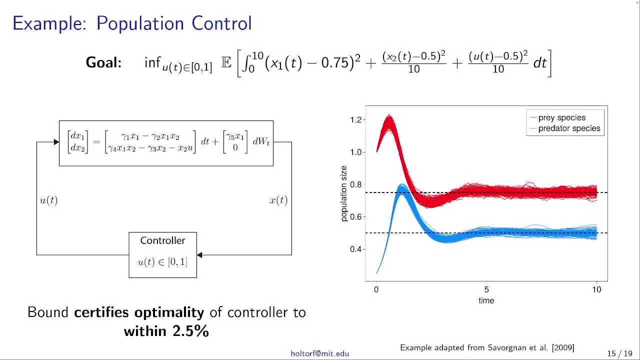 And what I found is that this controller- certainly that controller, I would say- passes the eyeball test. It drives the population sizes pretty quickly to the desired reference values and holds them there. And what's particularly interesting about this approach is that, because we have this lower bounding information, 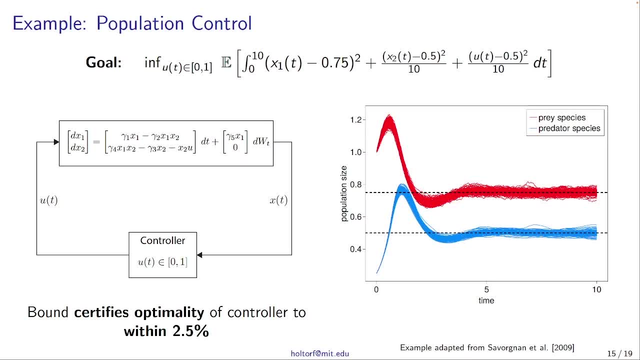 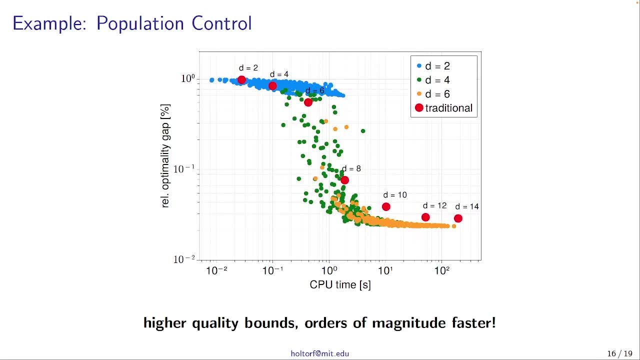 available as well. we can actually certify that this controller is no more than 2.5% suboptimal. So what's also interesting about this problem is that it showcases quite nicely that this partitioning idea that I talked about earlier can actually be hugely beneficial. 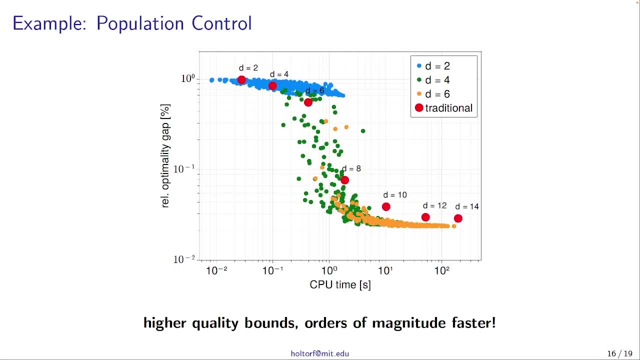 to the lower bounding problems In particular. this figure here shows the relative optimality gap comparing the performance of the best known controller to the lower bound obtained by these bounding problems, versus the time it took to solve these problems. So the big red markers here show the traditional approach. 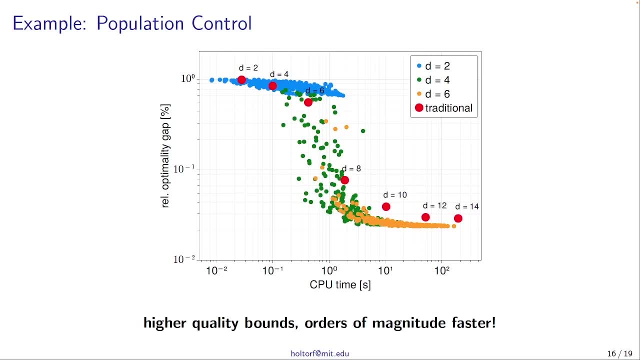 where we are looking for a global polynomial underestimator to the value function and where we improve our approximation, quality and bound simply by increasing the degree of that polynomial. The small markers instead show what happens when we optimize over a piecewise polynomial, for example for the partition of the problem domain. 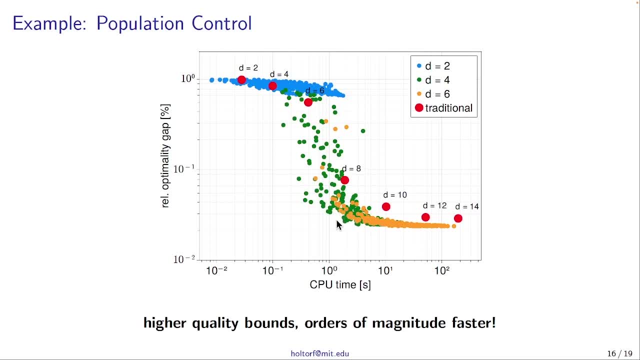 and, for a degree, of the polynomial pieces as color coded, And what this shows is that when we partition the problem domain suitably, we can actually compute better bounds than with the traditional approach, and we can do it orders of magnitude faster at the same time. 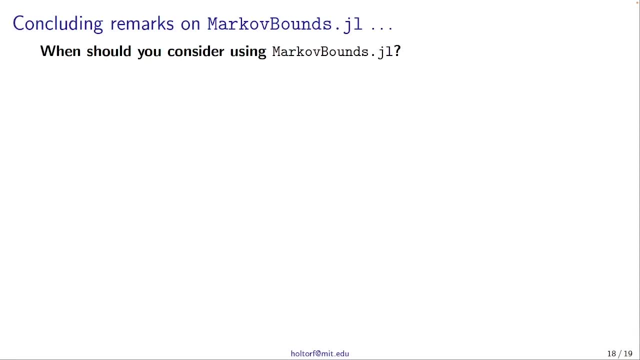 So, to conclude, I would like to briefly talk about when you should consider using MarkovBoundsjl. So, in particular, there are two conditions that are essentially non-negotiable. The first one is that you're working with a continuous time jump diffusion process.